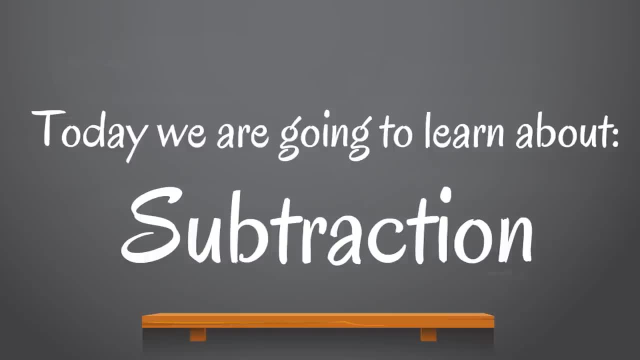 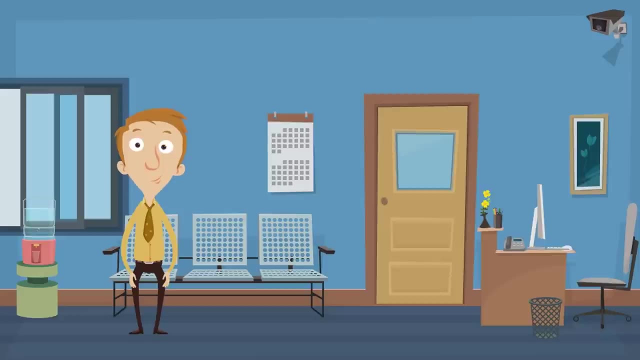 Today we are going to learn about subtraction. Oh, you know where I am. Yeah, you know. I'm waiting patiently in this waiting room. Oh man, it has been a while. Have you ever been in a waiting room before? Cool, Yeah, they can be fun, but you do have to be patient. and it's a good time to think. 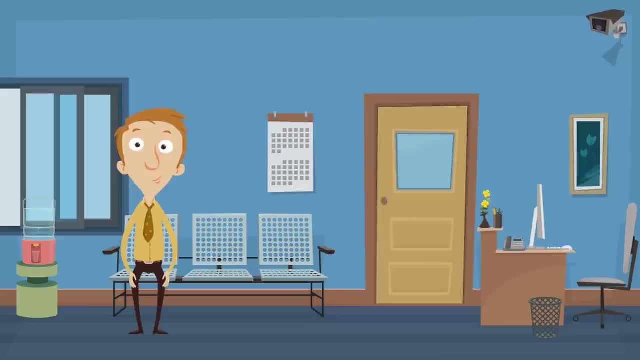 You know, you can think about all kinds of things, Like: okay, I have eight cowboy hats. I know it's crazy, it's weird: eight cowboy hats and they're all the exact same, The exact same hat. I've got eight of them, Eight brown. 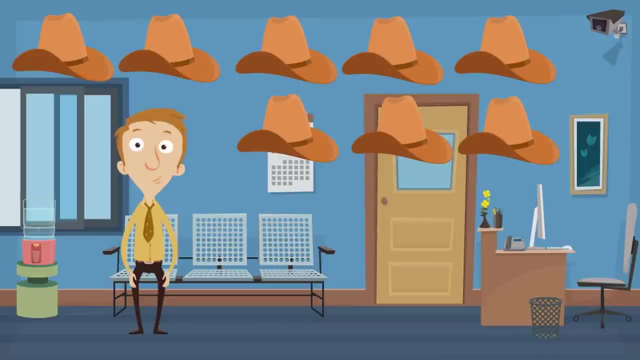 cowboy hats. I mean, what's a guy going to do with eight brown cowboy hats that look the exact same? What could I possibly do with eight brown cowboy hats that are all the same? I mean, I should probably give some of them away. You know, I could give away. 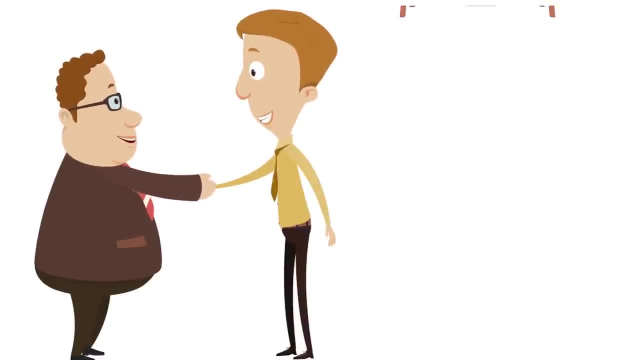 one of my hats to Bob, And Cookie might want one. Yeah, she might like a brown cowboy hat. you know I could give one to Nick Nancy, you know, just in case she ever got invited to a western party And Chomsky he'd. 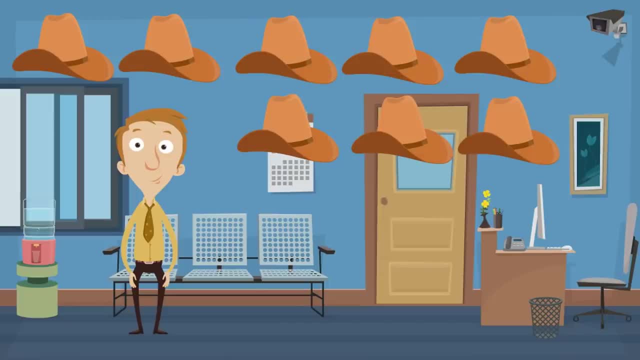 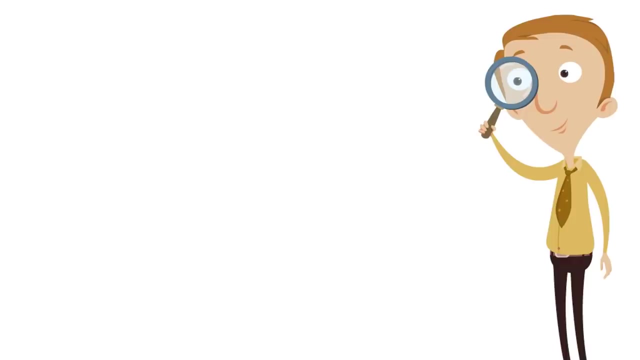 take a hat. So as I'm sitting here thinking about my eight hats, I need to figure out how many hats I'll have left if I give some of them away. To figure that out, we need to use subtraction. You see, subtraction is when you take numbers away. Yeah, very simple. Subtraction is when 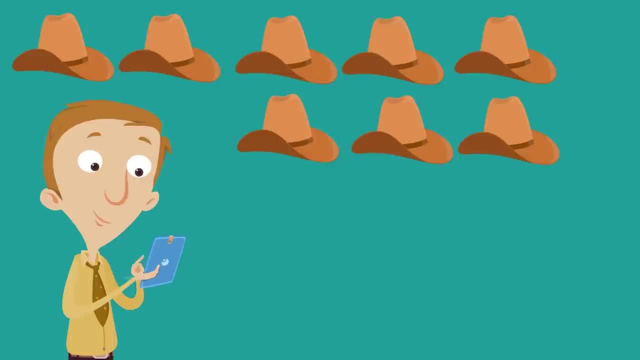 you take numbers away, Subtraction. So I begin with eight hats And I decide to give one away. We're going to need to subtract one from eight. The way we would write this is eight minus one. Now remember, when we subtract we're just taking numbers away. So eight minus one. 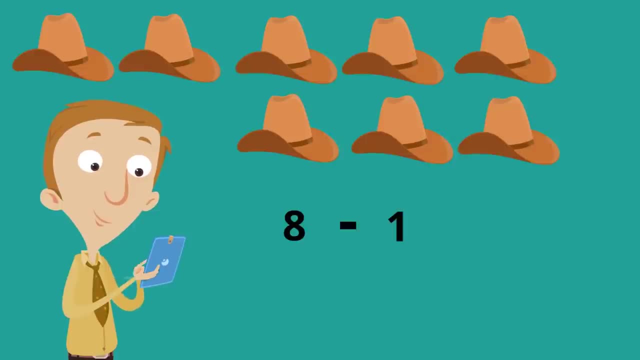 we're going to just take one away. There we go. How many hats do I have left? What is 8 minus 1?? If it helps, you can just count how many hats I have left. What is 8 minus 1?? 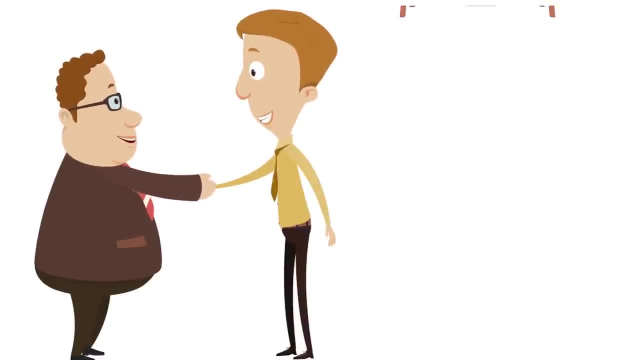 one of my hats to Bob, And Cookie might want one. Yeah, she might like a brown cowboy hat. you know I could give one to Nick Nancy, you know, just in case she ever got invited to a western party And Chomsky he'd. 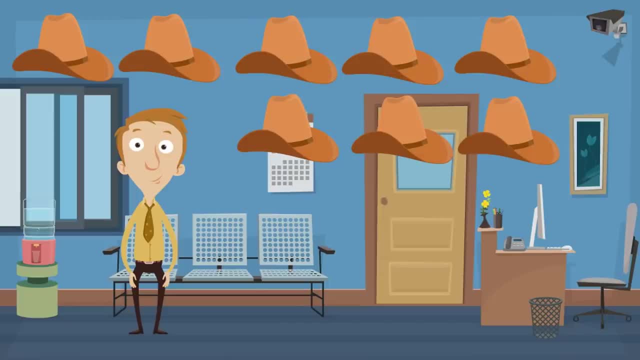 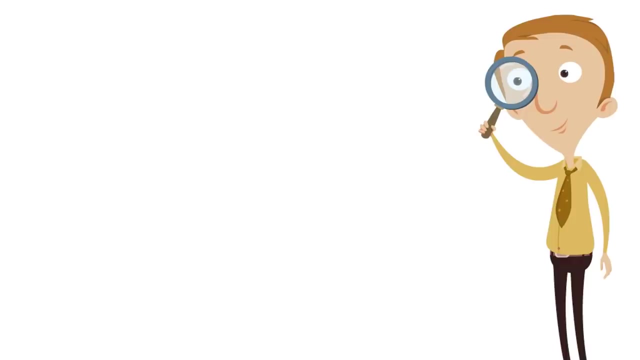 take a hat. So as I'm sitting here thinking about my eight hats, I need to figure out how many hats I'll have left if I give some of them away. To figure that out, we need to use subtraction. You see, subtraction is when you take numbers away. Yeah, very simple. Subtraction is when 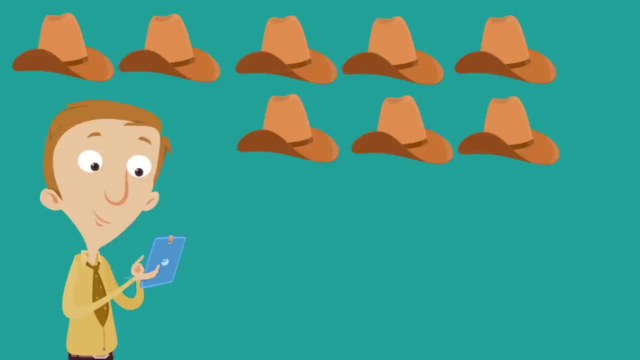 you take numbers away. So I begin with eight hats and I decide to give one away. We're going to need to subtract one from eight. The way we would write this is eight minus one. Now remember, when we subtract we're just taking numbers away. so eight minus one we're going to 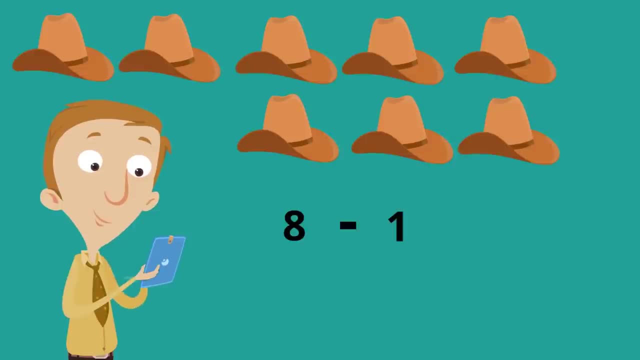 just take one away. There we go. How many hats do I have? They can't do more thanную. Yeah, There we go. That's what we need, And I'm gonna subtract another eight from this one and it gets a number. 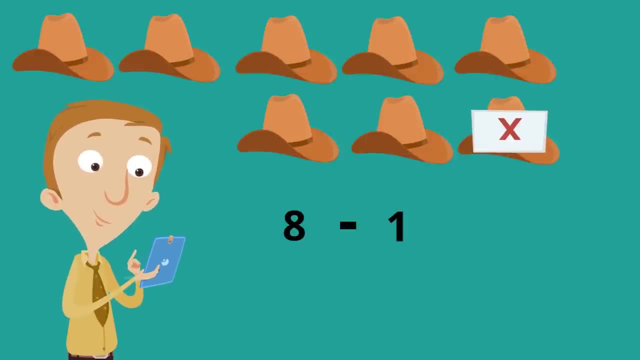 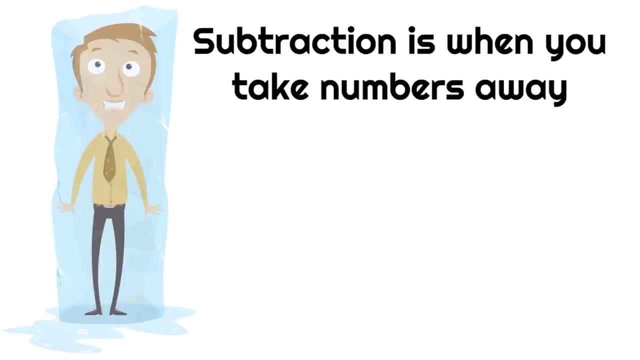 do I have left? What is 8 minus 1?? If it helps, you can just count how many hats I have left. What is 8 minus 1?? Yeah, 7.. 8 minus 1 is 7.. Now I have 7 hats Remember. 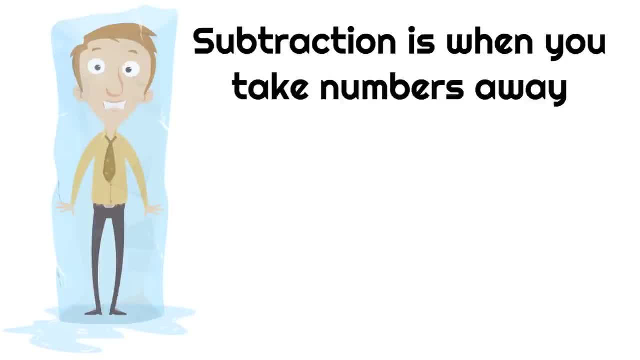 subtraction is when you take numbers away And, as you might have noticed, we use the minus sign when we write a subtraction problem. You can see it right there in the middle. It's just like a dash. That's the minus sign. So now I have. 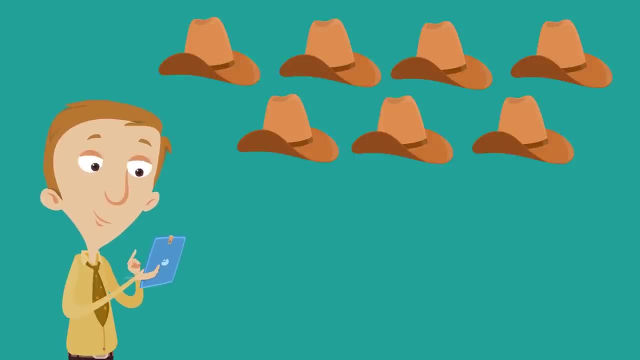 seven hats. but two of my friends stopped by and I decide: you know what? I know I just have seven hats now, but I want to give two of them away. Now I'm gonna be subtracting two hats from my collection. We would write this by saying 7 minus 2.. 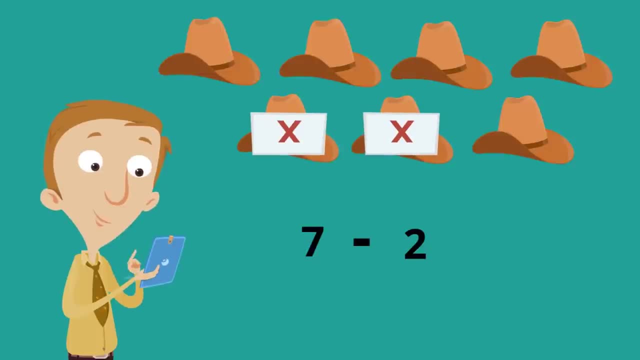 Now let's take away two hats. We'll find out how many we have left. What a wonderful subtraction problem. What is 7 minus 2?? If you need help, you can just count how many hats are left. What is 7 minus 2?? 7 minus 2 equals. 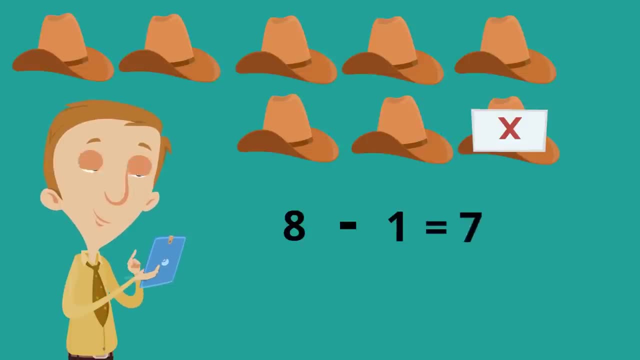 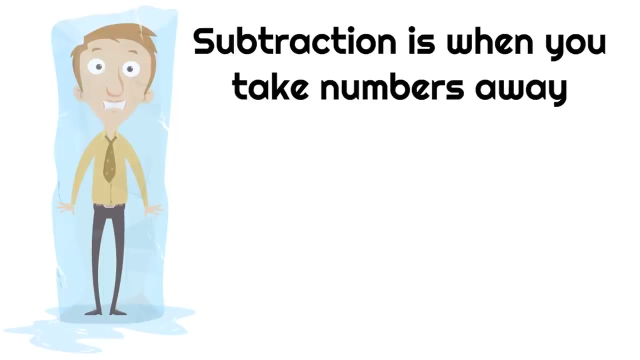 Yeah, 7.. 8 minus 1 is 7.. Now I have 7 hats. Remember, subtraction is when you take numbers away And, as you might have noticed, we use the minus sign when we write a subtraction problem. You can see it right there in the middle. 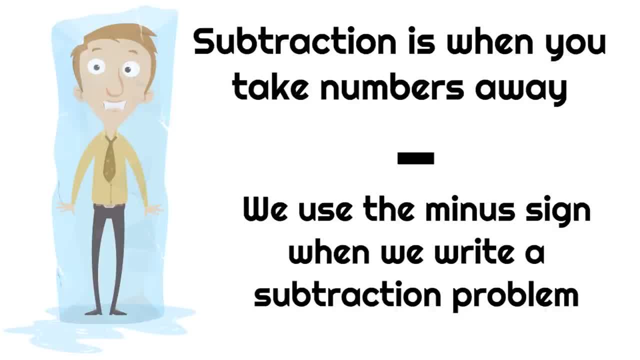 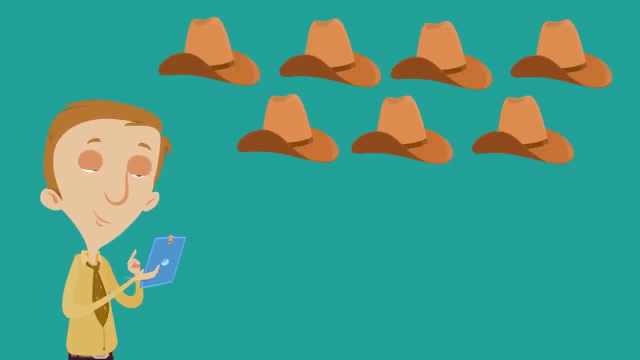 It's just like a dash. That's the minus sign. So now I have 7 hats, but two of my friends stop by and I decide: you know what? I know, I just have 7 hats now, but I want to give two of them away. 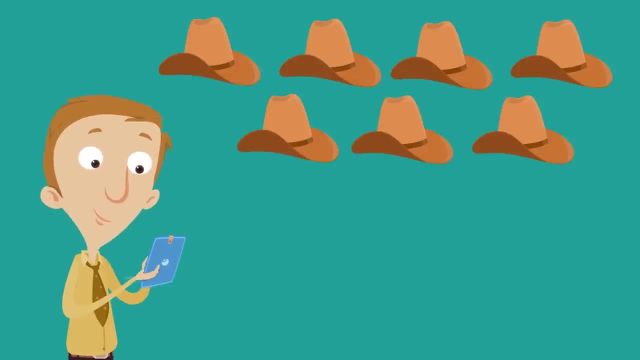 Now I'm going to be subtracting two hats from my collection. We would write this by saying 7 minus 2.. Now let's take away two hats, We'll find out how many we have left. What a wonderful subtraction problem. What is 7 minus 2?? 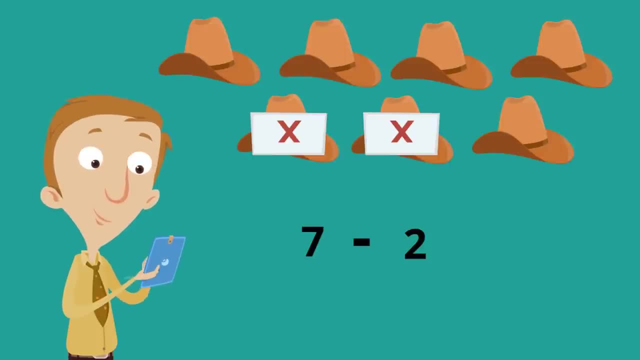 If you need help, you can just count how many hats are left. What is 7 minus 2? 7 minus 2.. 7 minus 2 equals 5, yeah, 5 hats. and you can even count them: 1,, 2,, 3,, 4,, 5, there. 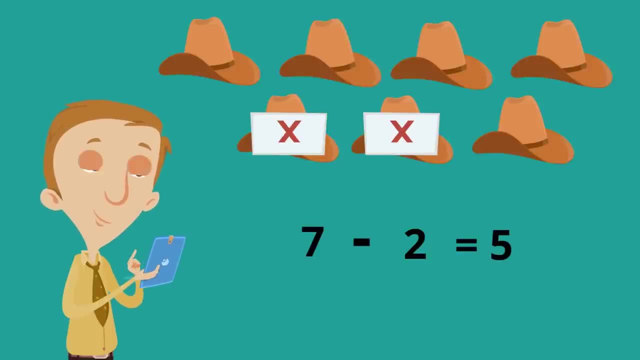 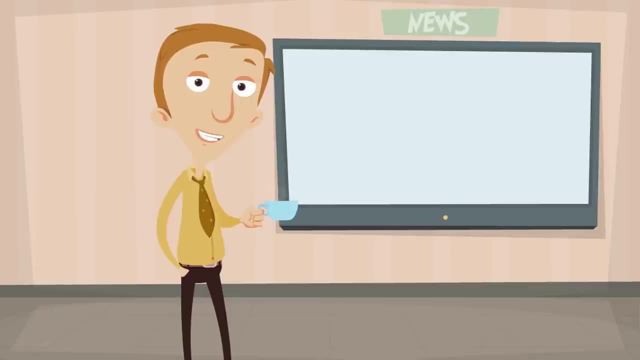 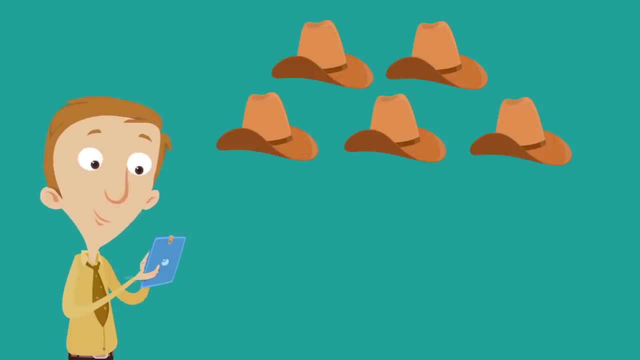 are 5 hats left. 7 minus 2 equals 5.. Do you see how fun and simple subtraction is? Subtraction is when you take numbers away. So now I have 5 hats in my collection. only 5 hats left. 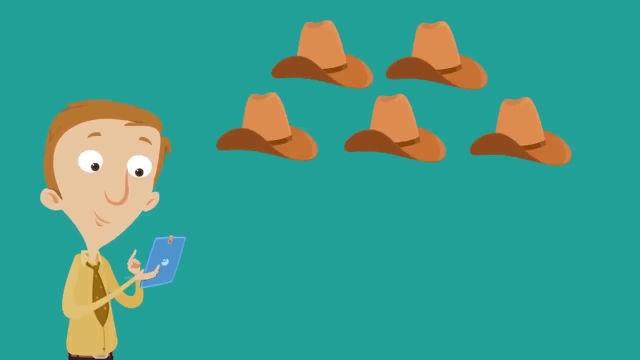 But then I meet up with my cousins Hooey, Dewey and Stewie, who want to have hats too, and I'd love to give them hats. So I'm going to give 3 more hats away. So I have 5 hats and we're going to subtract 3 hats. 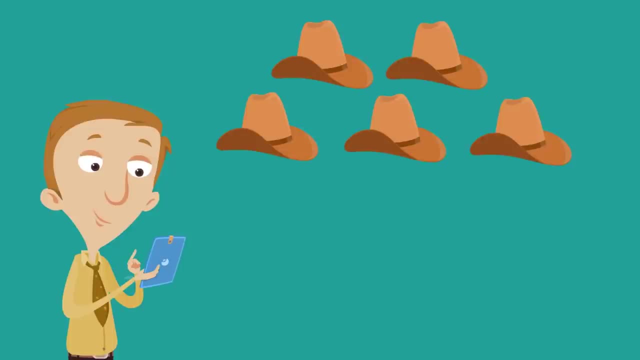 We would write that 5 minus 3.. Oh, I love subtraction so much. All right, bada bing, there we go. The 3 hats are gone. So 5 minus 3, how many hats are left? It's pretty simple, isn't it? 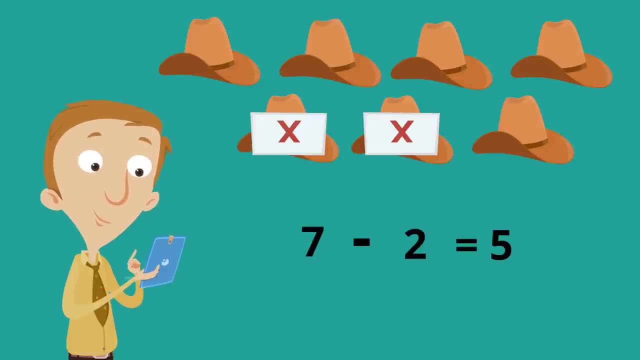 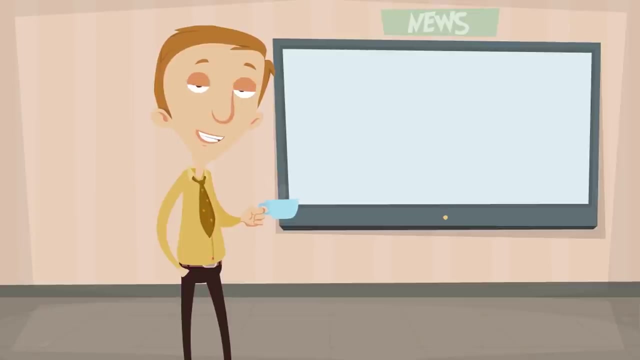 Five, Yeah, Five hats, And you can even count them: One, two, three, four, five. There are five hats left. Seven minus two equals five. Do you see how fun and simple subtraction is? Subtraction is when you take numbers away. 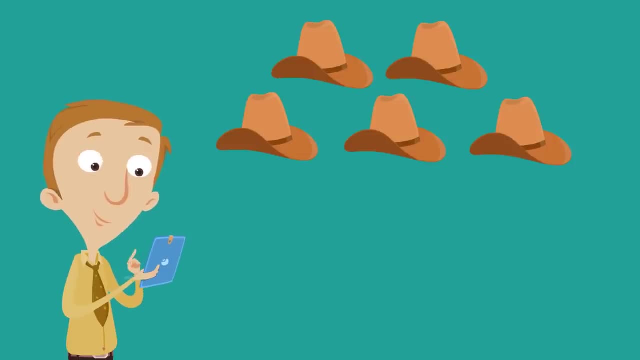 So now I have five hats in my collection- Only five hats left. But then I meet up with my cousins Hooey, Dewey and Stewie, who want to have hats too, And I'd love to give them hats. So I'm going to give three more hats away. 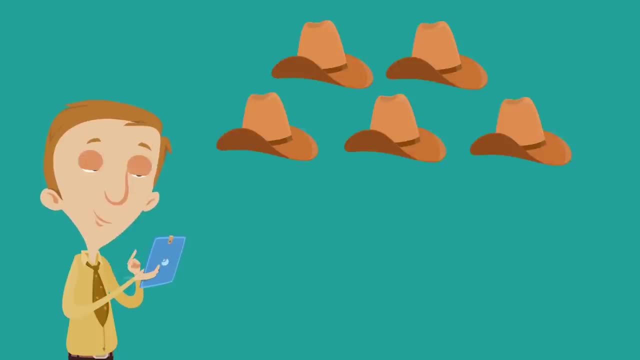 So I have five hats and we're going to subtract three hats. We would write that five minus three. Oh, I love subtraction so much. All right, Ba-da-bing, There we go. The three hats are gone. So five minus three. how many hats are left? 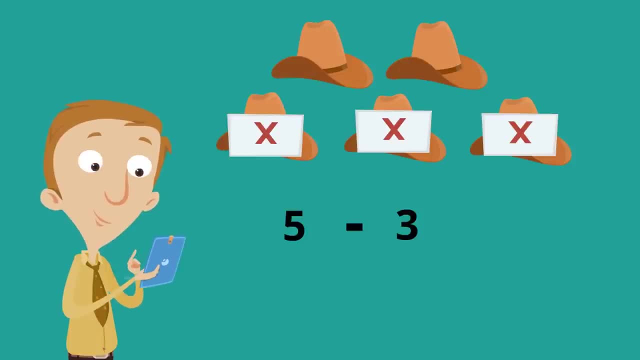 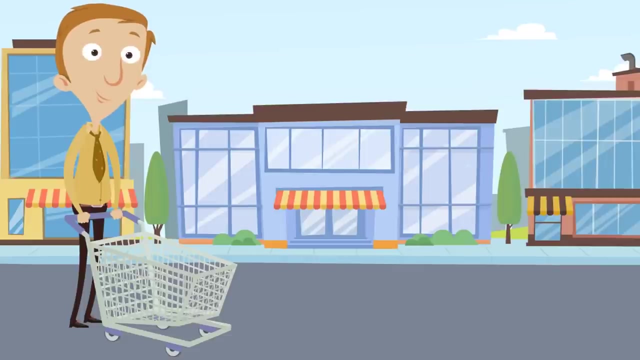 It's pretty simple, isn't it? Yeah, Five minus three equals two. Good job. Subtraction is just taking numbers away, And five minus three leaves you with two. Now I have just two hats. We love subtraction. I mean, subtraction is when you take numbers away. 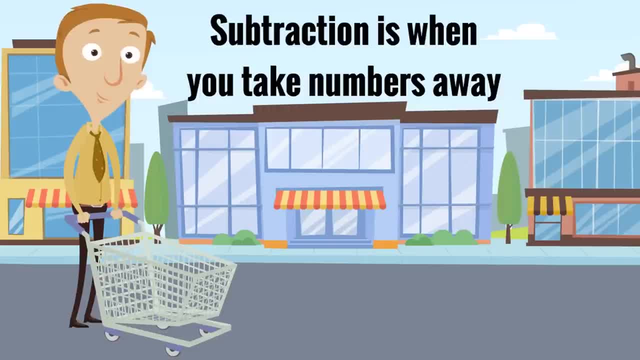 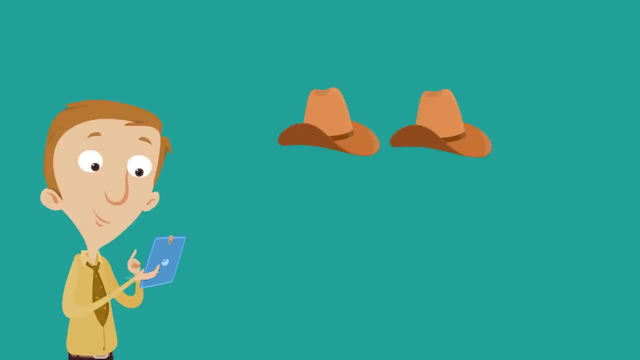 And why am I in the middle of the road with a shopping cart? Ha ha. So I have my two hats and that's fun, because then the hat has a friend and they're like buddies and they're like a pair of. 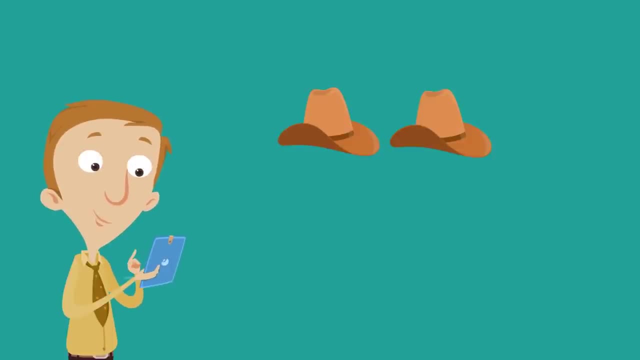 a pair of a pair of friends. and then Chomsky came by and I said, oh, I'm going to have to do subtraction again, I'm going to have to subtract again. Oh, Chomsky, you know that, Choms, he came by. 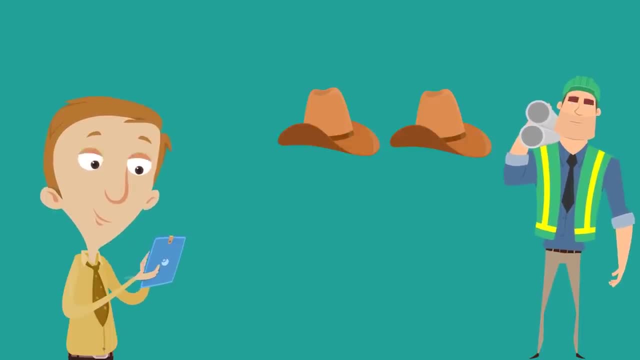 I said I'm going to have to subtract again, I'm going to have to subtract one more time. Subtraction again, Subtraction again, Subtraction again. So I have two hats Minus one, Two minus one. So we subtract that one, we take that one away, and how many hats are left? 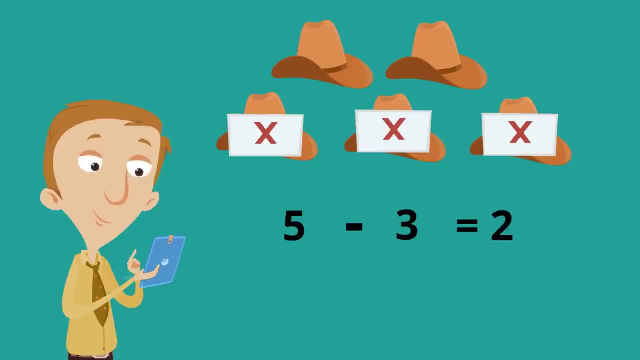 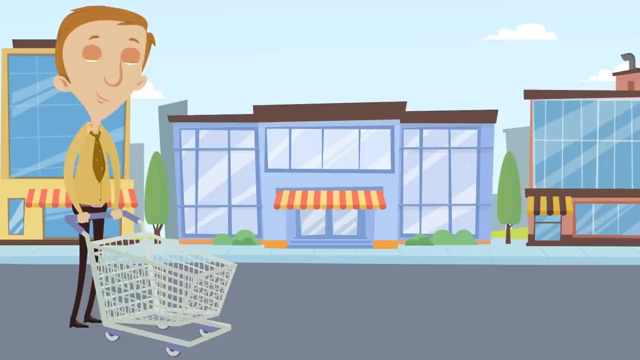 Yeah, 5 minus 3 equals 2.. Good job, Subtraction is just taking numbers away, and 5 minus 3 leaves you with 2.. Now I have just 2 hats. We love subtraction. I mean, subtraction is when you take numbers away. 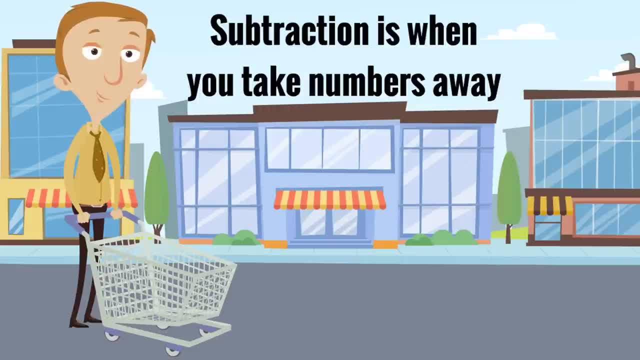 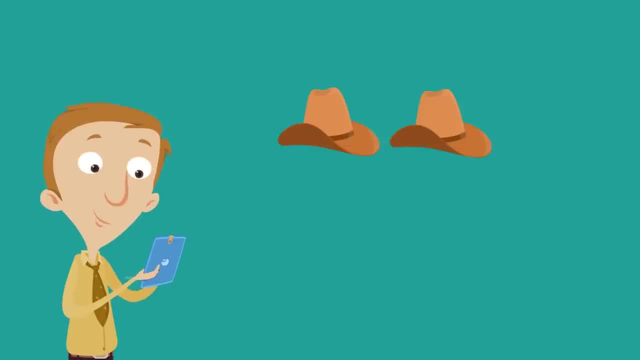 And why am I in the middle of the road with a shopping cart? So I have my 2 hats and that's fun, because then the hat has a friend and they're like buddies and they're like a pair of friends. and then 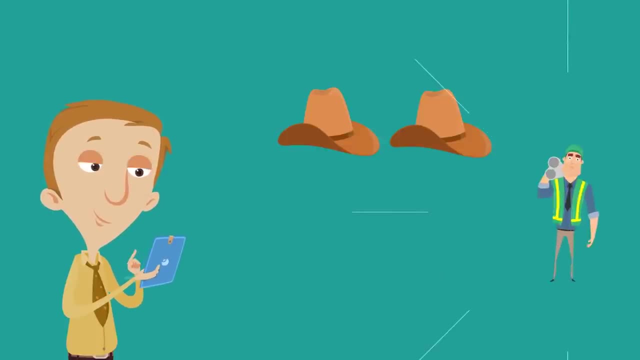 Chomsky came by And I said, oh, I'm going to have to do subtraction again. I'm going to have to subtract again. Oh, Chomsky, you know that Chomsky came by. I said I'm going to have to subtract again. 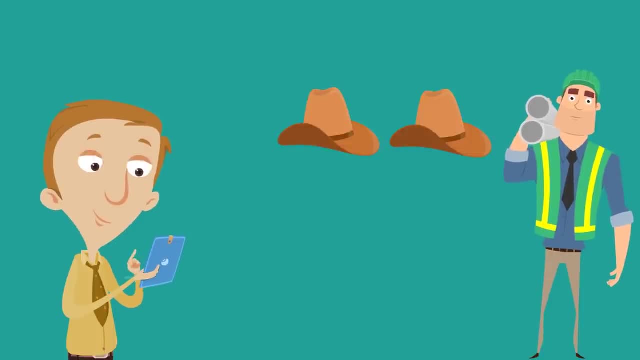 I'm going to have to subtract one more time. So I have 2 hats minus 1.. 2 hats, 2 hats, 2 hats minus 1.. So we subtract that one and we take that one away, and how many hats are left? 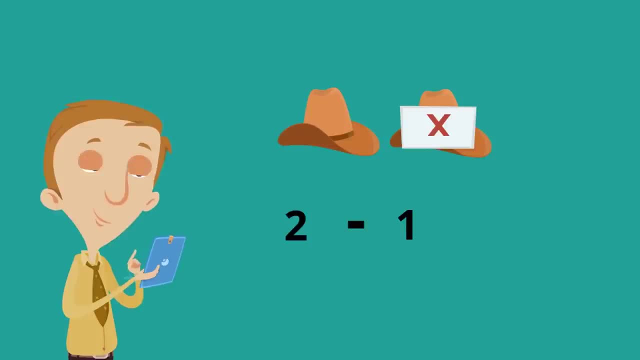 What is 2 minus 1?? Yup, 2 minus 1 equals 1.. There's only one hat left, Which is fine. I mean, you know, I can only wear one hat at a time, And it was the same exact hat. 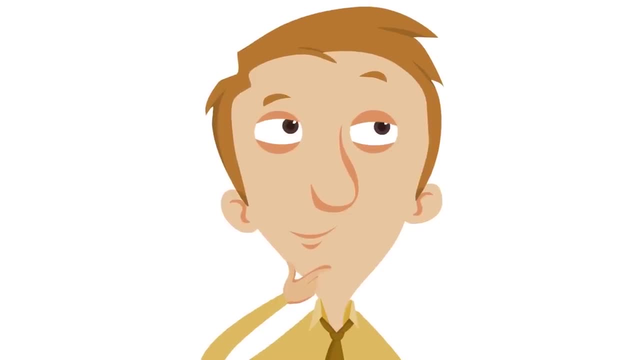 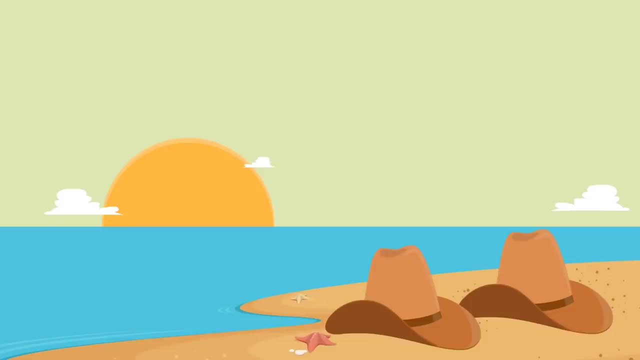 Oh, okay, I think about it. Subtraction's been good to me. It's good. Subtraction is taking numbers away. Sometimes I do wonder what would have happened if I didn't give that hat away. If Hattie still had his friend, they could have gone to the beach together. 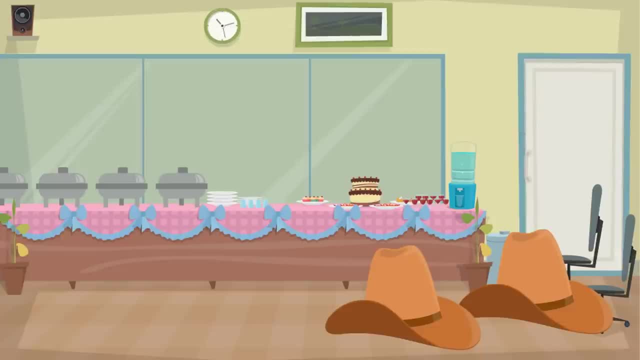 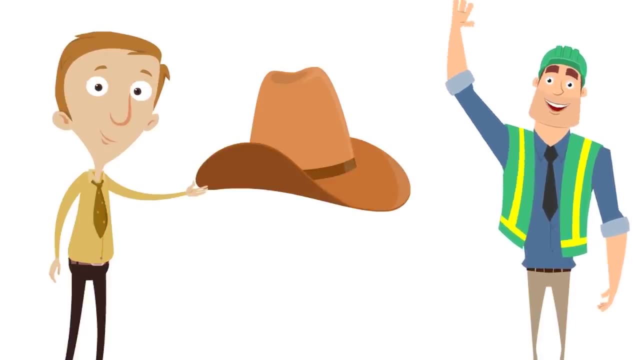 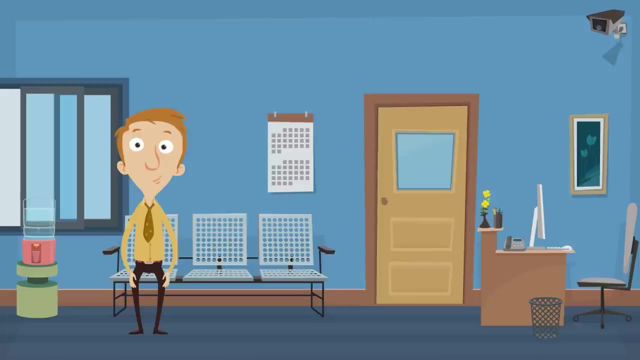 They could have gone to birthday parties together, But actually the hat had a better purpose: To make a friend happy. So in this waiting room all I gotta say is: thanks, Subtraction, You are pretty awesome.